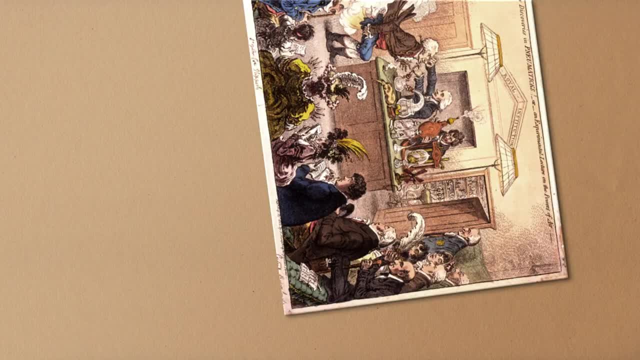 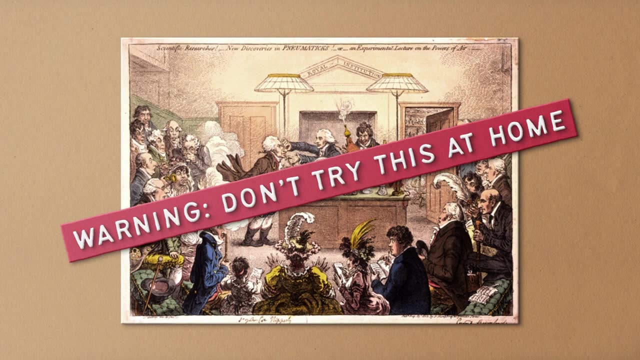 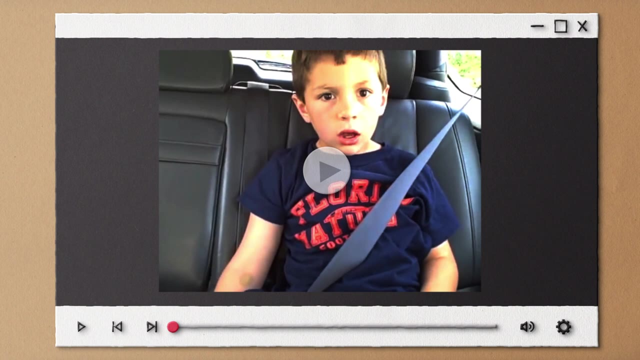 use of nitrous oxide. As you may imagine, these experiments were not up to the scientific standards that they were supposed to have. They were only used for the use of nitrous oxide. In fact, it would be accurate to say that those experiments were conducted in a similar fashion. 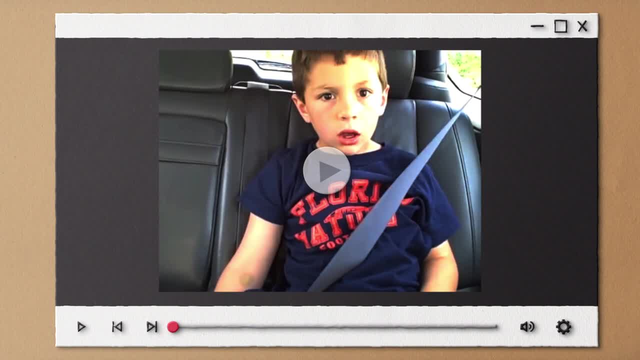 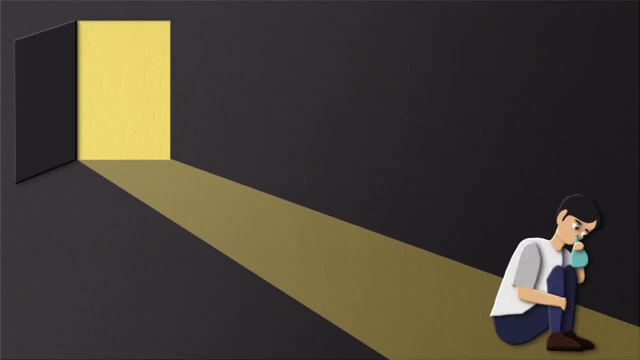 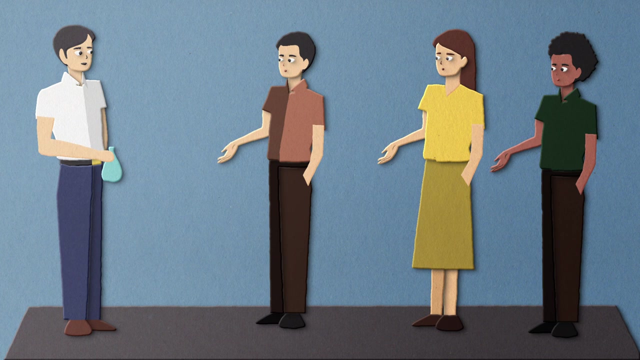 as the popular YouTube clip David After Dentist In 1799, Davy took the gas outside of laboratory conditions, inhaling vast amounts of it in solitary sessions in the dark. He also started offering the gas to healthy subjects, usually his friends and family, and asked them. 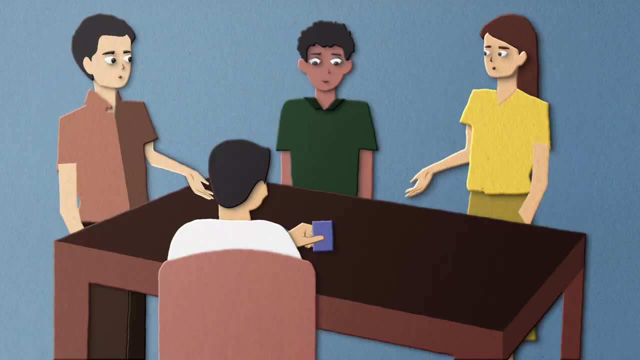 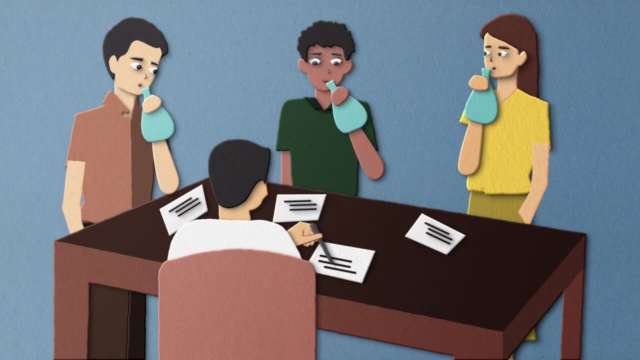 to write down their experiences. Well, when I get together with friends, I like to play a board game, but apparently Davy preferred drugging up his friends' and writing reports. well, to each their own. We still don't exactly know how nitrous oxide works on the brain and body. 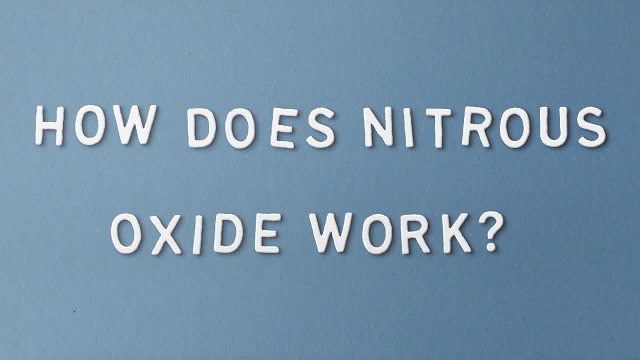 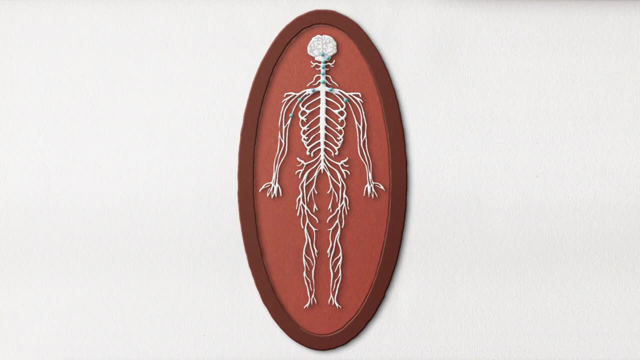 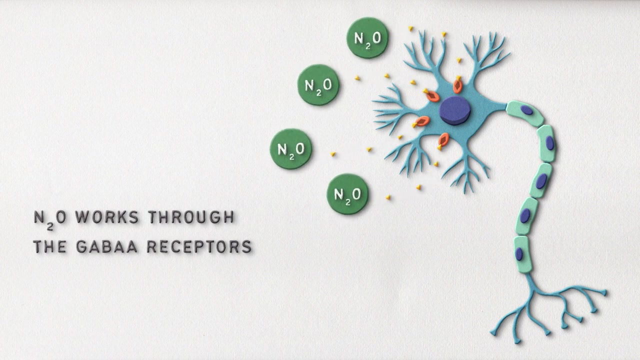 but scientists have a few theories regarding the physiological mechanisms. Simply put, it is believed that nitrous oxide impacts how neurotransmitters send pain signals around the body. N2O works through regulated ligand-gated ion channels in the body, the GABA receptors, which control a big portion of inhibitory signaling in the nervous system. 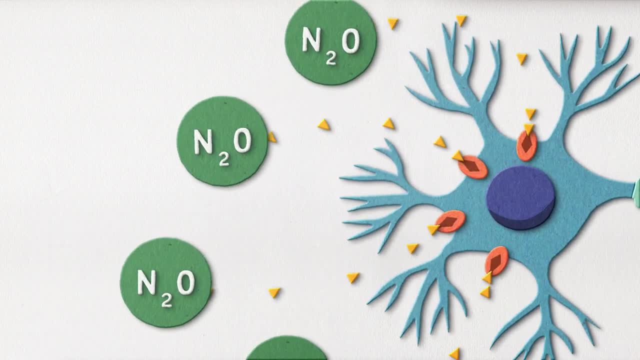 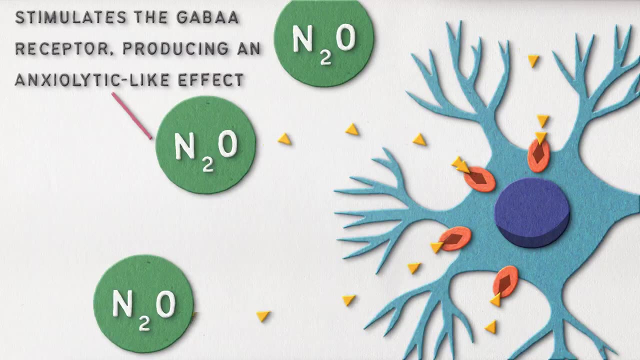 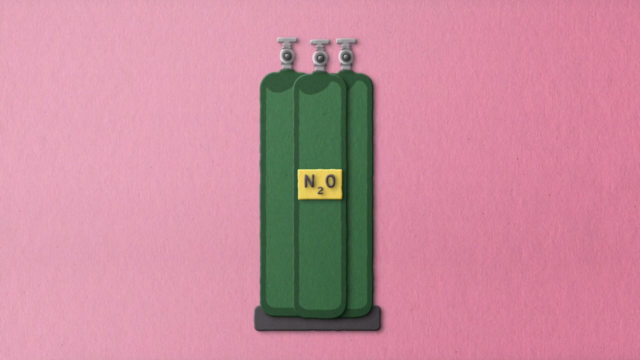 Similarly to other anesthetics such as benzoyl benzodiazepines, N2O stimulates the GABA receptor, producing an anxiolytic-like effect. Another popular hypothesis is that the N2O-induced analgesic effect could be similar to that of 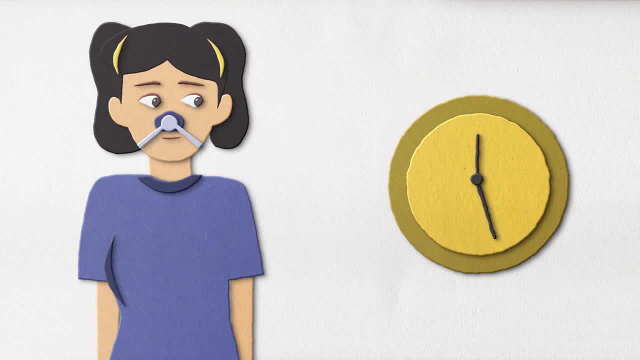 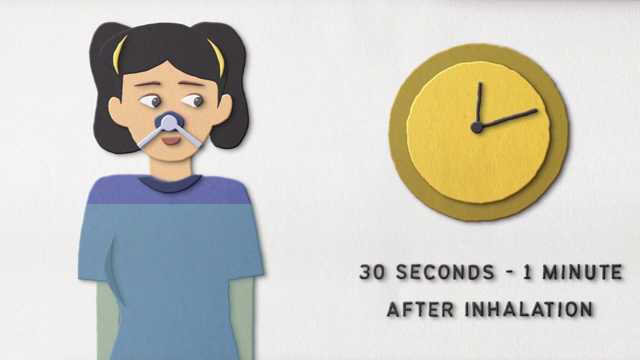 the opioids like morphine. When it comes to the effect nitrous oxide has on your body, that will depend on how much you inhale and for how long. Typically, you start to experience the effects within 30 seconds to one minute after inhalation, and the effects wear off within. 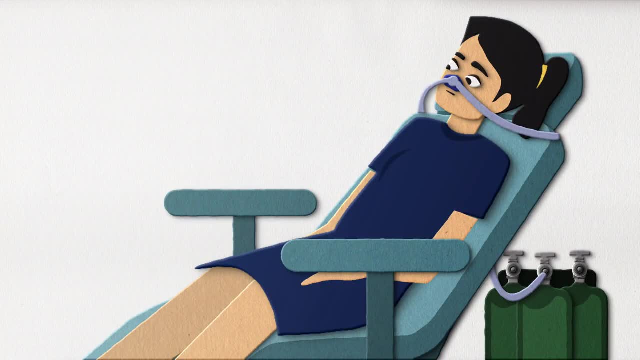 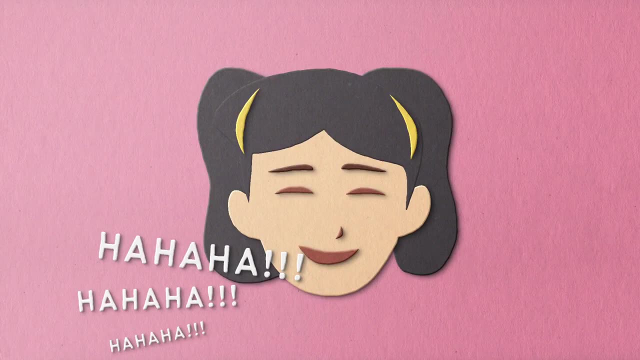 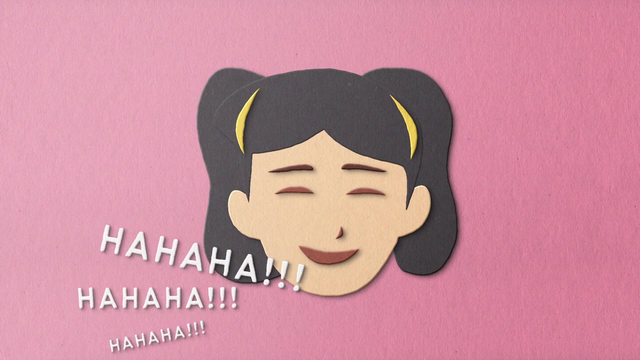 minutes after you cease inhaling. This is why it is necessary that the patient continually inhales the gas during a medical procedure. But what do people actually experience when, under the effect of laughing gas, Do they really start giggling or seeing things that weren't there in the first place? As a matter of fact, some people 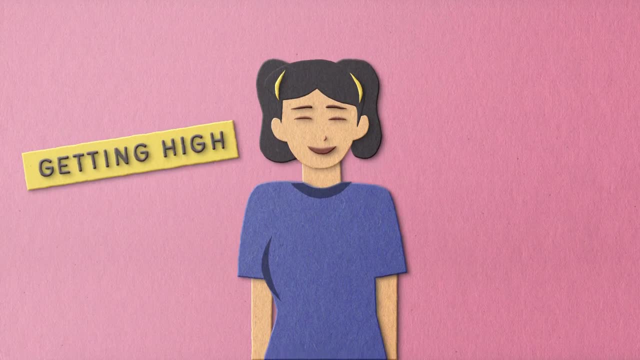 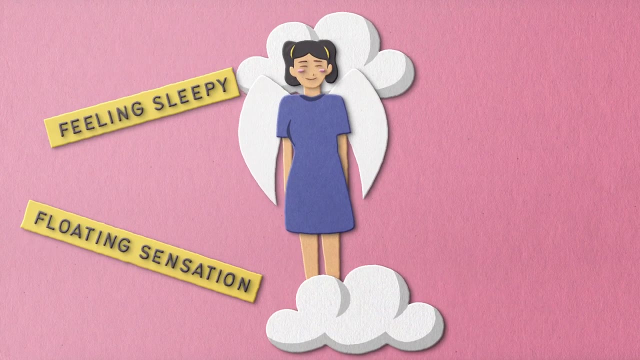 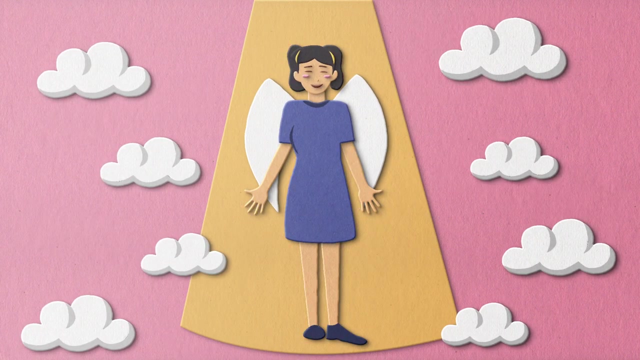 have described similar sensations to getting high, like feeling lightheaded, experiencing a floating sensation, feeling sleepy or even tingling in their arms and legs. Those effects can create a feeling of euphoria and relaxation that will make you more prone to laughing and be less aware of. 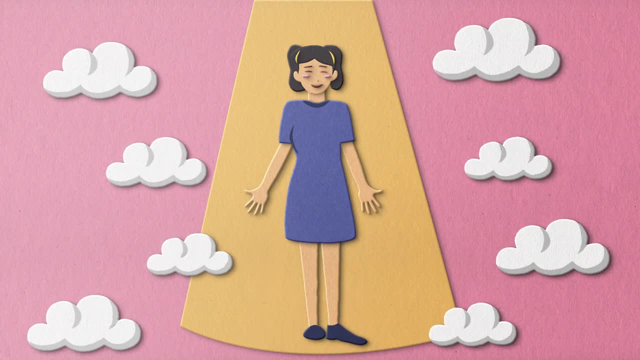 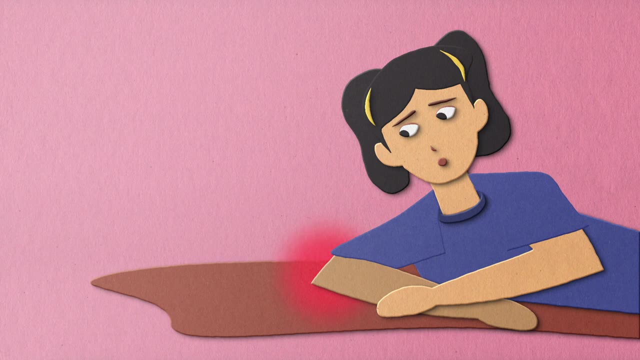 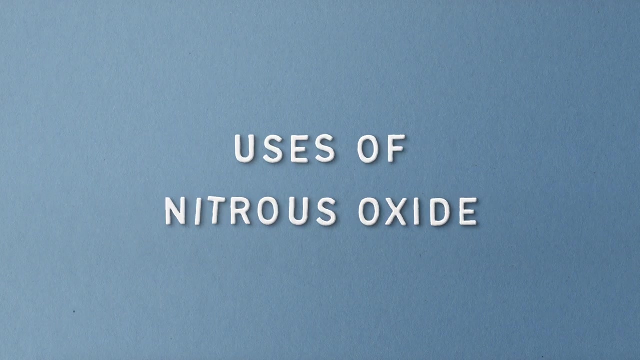 your fears and things that make you anxious. N2O does also have an analgesic effect, but it is important to mention that although N2O helps dull the pain, it does not eliminate it completely. Now that we know what nitrous oxide is, let's find out where we use it. One of the common uses: 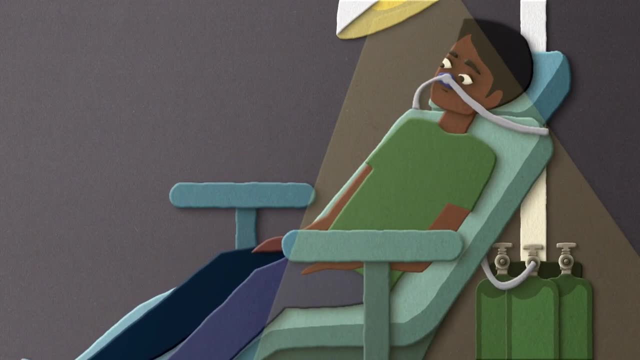 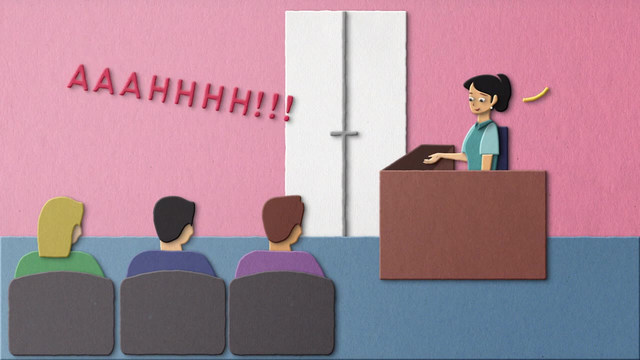 of nitrous oxide is, like we have mentioned at the beginning of this video, dentistry. Despite advancements in the field, many people still feel extremely anxious about attending dentist appointments and benefit from nitrous oxide's anxiolytic effects. Nitrous oxide. 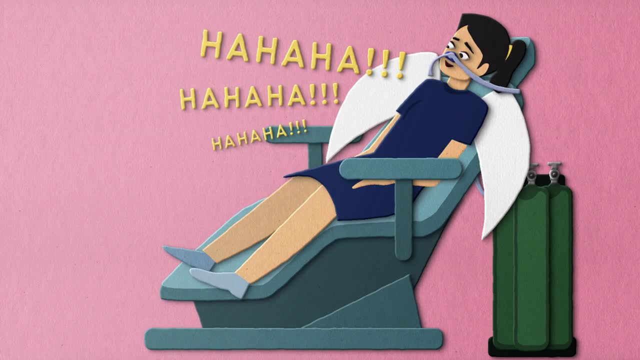 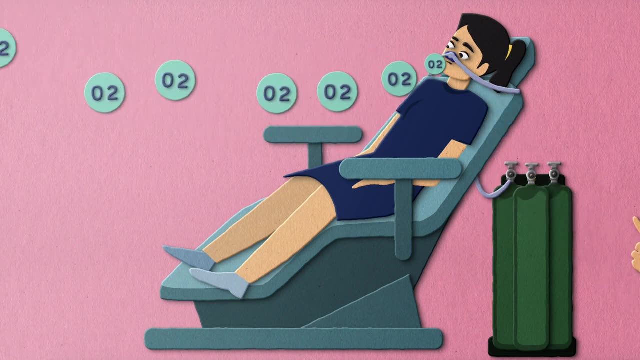 is commonly used in conjunction with oxygen, so if you start to feel the effects too strongly, the dentist can switch off the N2O and the effects will wear off quickly as you inhale oxygen. Headaches are also a common use of nitrous oxide. 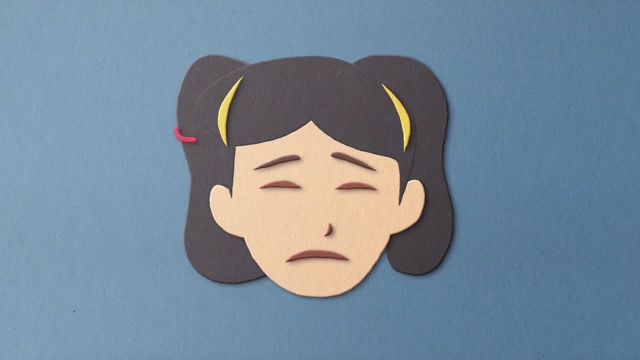 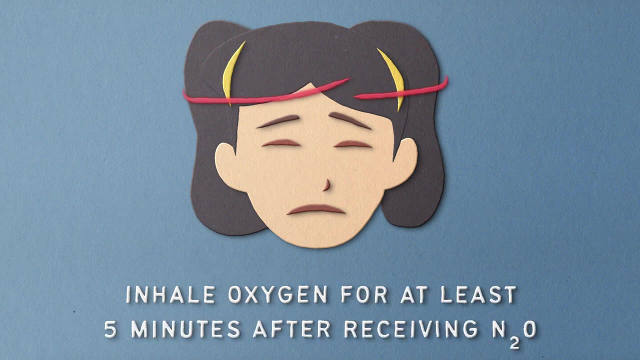 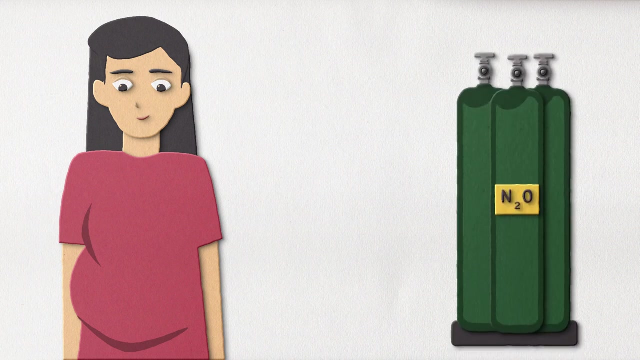 So many dentists require that you inhale oxygen for at least five minutes after receiving N2O to avoid a sore head. Nitrous oxide can be used in childbirth. In some countries, women can use nitrous oxide in labor to help alleviate painful contractions during childbirth. 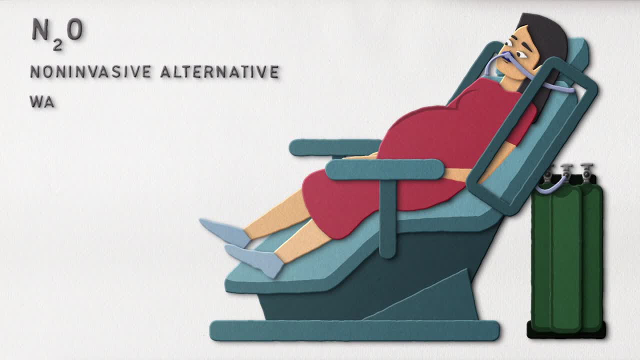 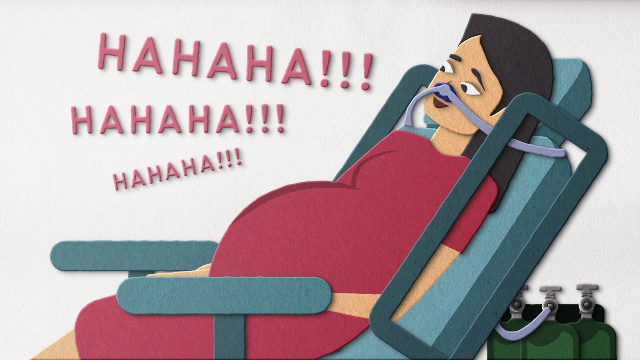 Nitrous oxide comes as a non-invasive alternative way of managing pain without restricting mobility. It can also be used to slow down labor or causing any harm to the baby. You're probably picturing women laughing while giving birth, but that's not the case at all. 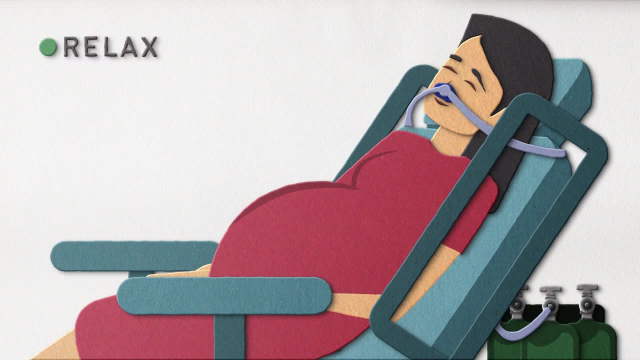 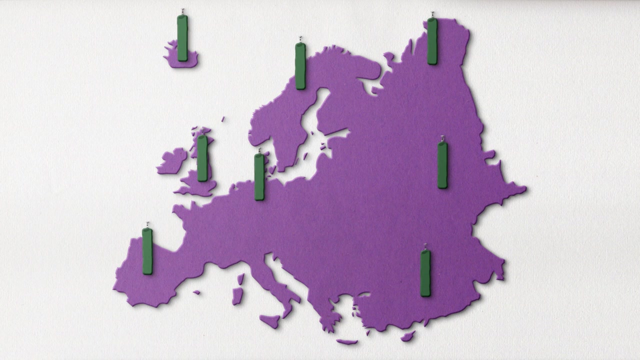 Laughing gas will only help the new mother to relax, relieve stress and anxiety and even allow her to move around, making labor a much more comfortable experience. The use of nitrous oxide in this setting is more prevalent in some countries than others. 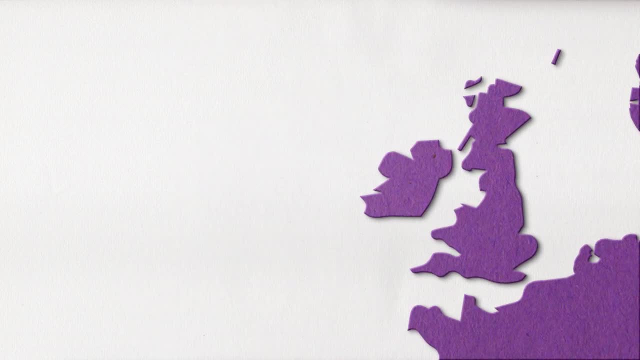 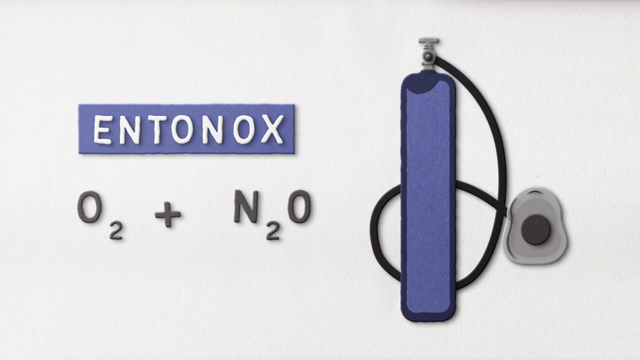 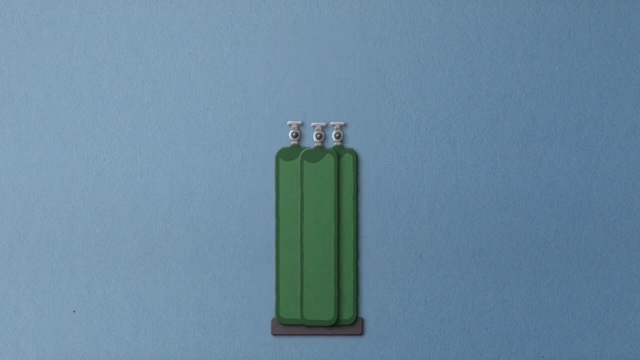 For example, in the UK it's commonly used in the form of Entonox. Entonox is a mixture of oxygen and nitrous oxide gas inhaled through a mask or mouthpiece. Nitrous oxide is also frequently used during childbirth in Finland, Canada, Australia. 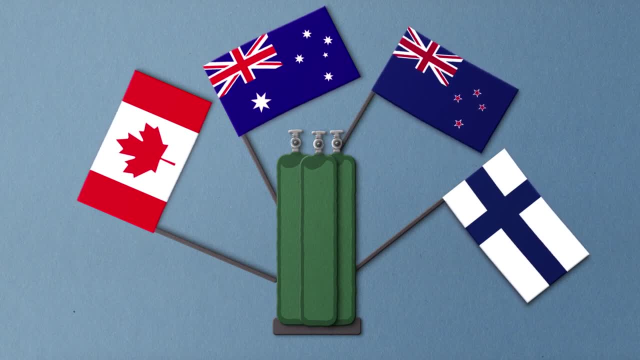 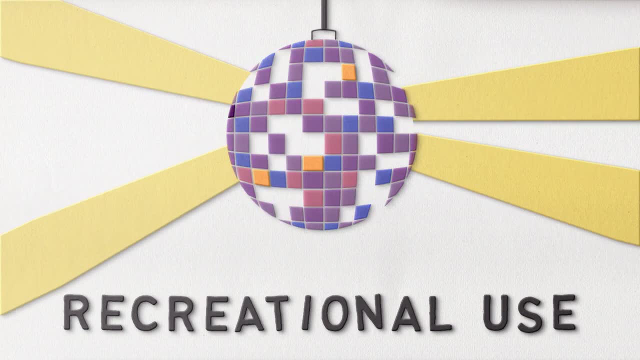 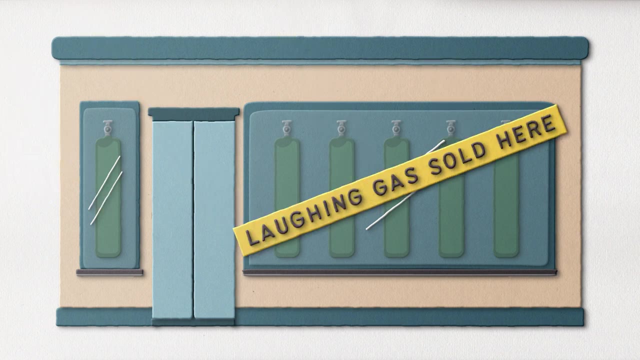 and New Zealand. The practice is less common in the US, but is growing in popularity every year. 4. DAVY WAS LISTENED IN THE US. Davey was not the only one using nitrous oxide recreationally. Today, in many countries the sale of N2O is not heavily restricted. 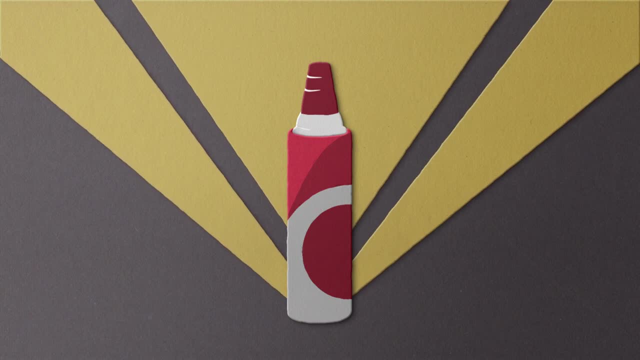 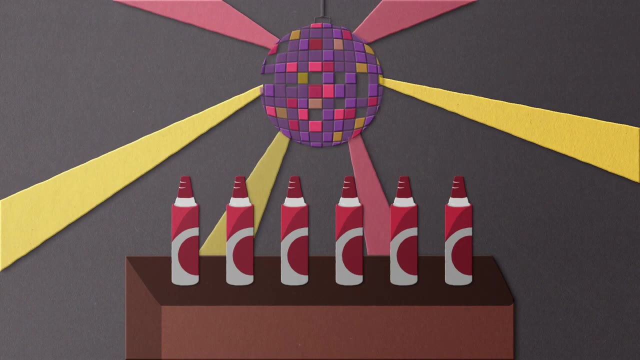 Typically nitrous oxide sellers don't advertise its recreational use but will promote N2O pressurized canisters to make whipped cream And looking at the data, you'd be forgiven for believing that partygoers have a passion for whipped cream. 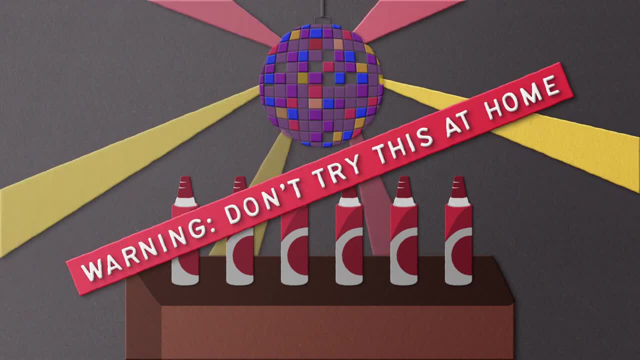 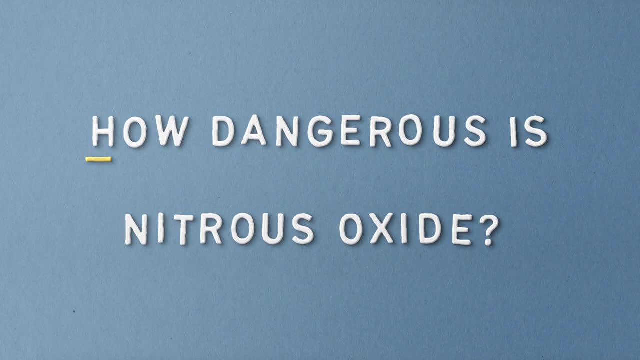 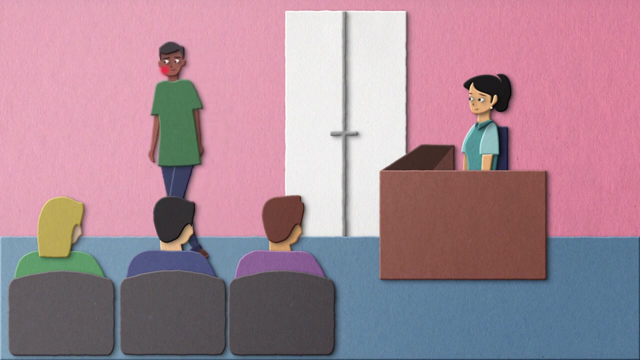 My advice: don't do it at home. Let your healthcare professional decide when you need laughing gas. Which brings me to the question: how dangerous is nitrous oxide? In a medical setting and with infrequent use, nitrous oxide is not dangerous and can make. minor medical procedures or events more tolerable. Sure, there could be, just like any other treatment, some common shortcomings, But it's not just about the short-term side effects like nausea, vomiting, dizziness and fatigue. However, medical professionals are able to supervise the administration of N2O. 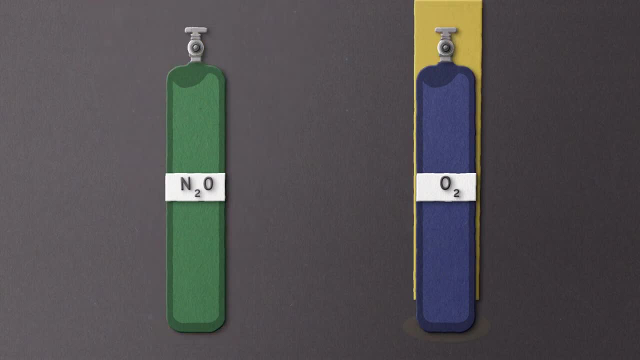 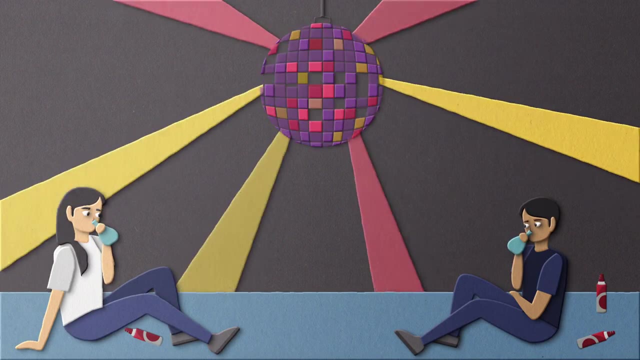 so that they can lower the risk of any adverse effects by restricting the flow of the gas or increasing the intake of pure oxygen. Nonetheless, there are some dangers associated with the recreational use of N2O. Just like any other drug, N2O's active and euphoric effects could cause you to act carelessly and dangerously. 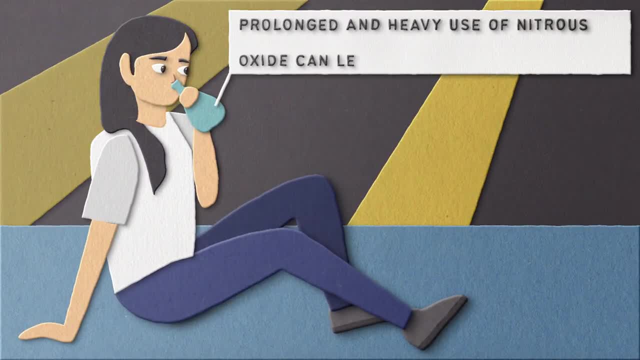 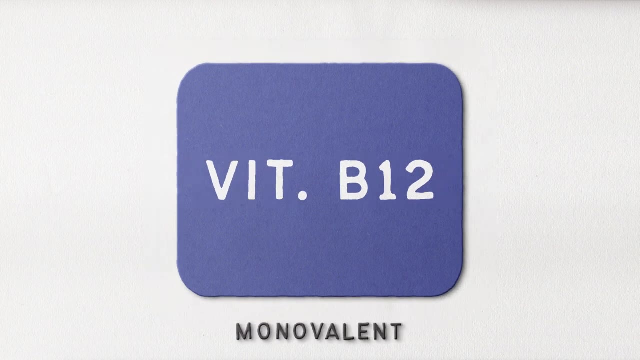 On top of that, prolonged and heavy use of nitrous oxide can lead to vitamin B12 deficiency, which in turn, can cause severe and irreversible nerve damage. And that happens due to the fact that N2O converts the active monovalent form of vitamin B12 to its 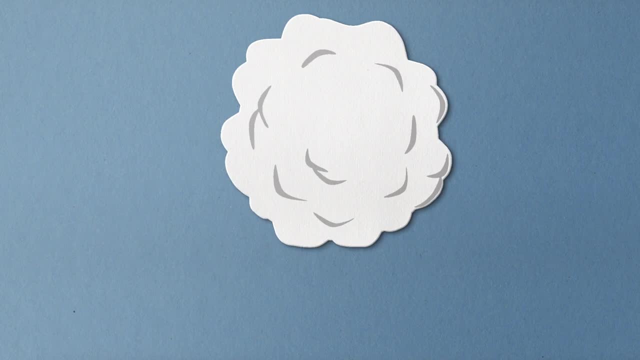 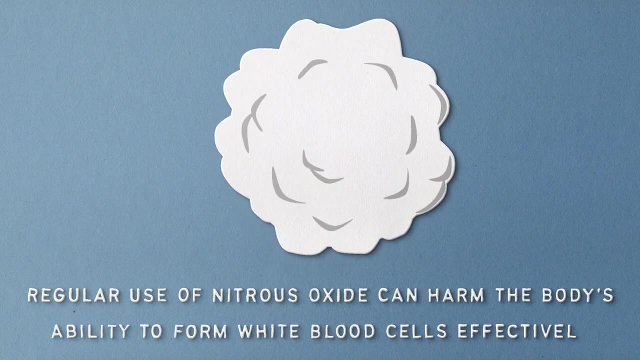 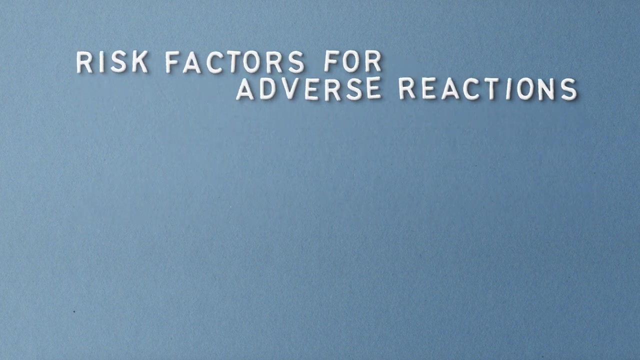 inactive bivalent form which your body can't use. It's also been reported that regular use of nitrous oxide can harm your body's ability to form white blood cells effectively. Similarly, there are also some medical conditions that could increase the risk of adverse reactions.